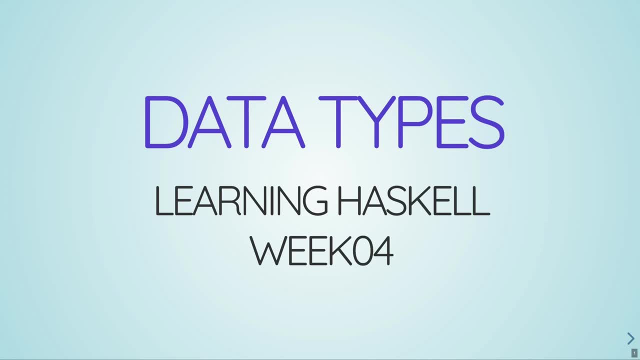 Welcome to my tutorial on data types. We've already seen pre-existing types in Haskell and hopefully you've learned a little bit about how they're important to Haskell and programming languages in general. Today, we're going to learn even more about them, partly by creating our own. 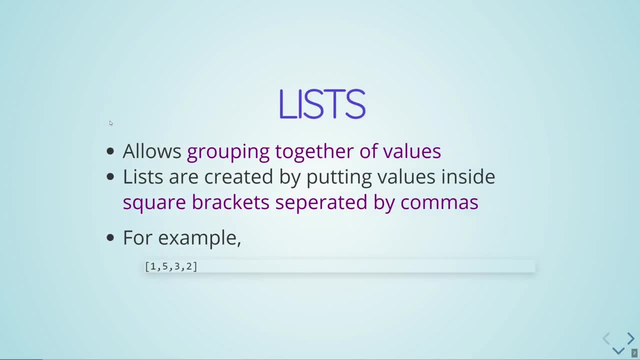 types. Before we get into that, though, let's talk a little bit about our favorite data type lists. So lists, you've already seen them. it's hard to do much work in Haskell without them. They allowed the grouping together of values using a special syntax, that are these square brackets and each element separated by a comma. 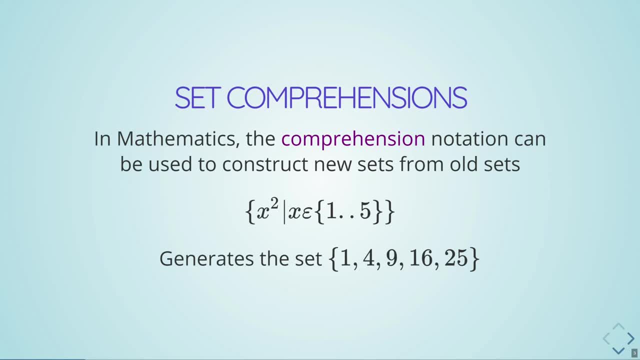 Set comprehension is a notation used in mathematics to specify sets in a dynamic sort of way. So usually it's done with either a vertical bar like this or some sort of like dot, and what you do is you specify the set with curly braces. usually in math we use curly braces to 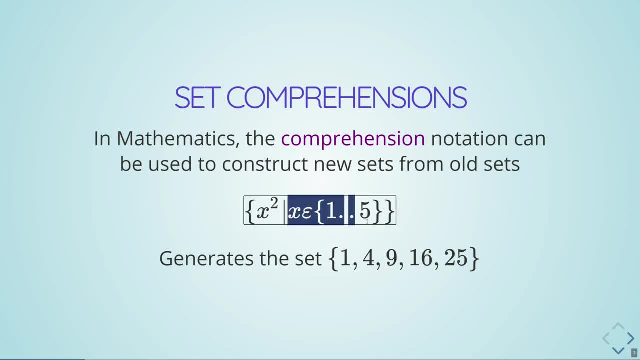 specify sets, and what you do is you specify what you call a generator- this part here- and you say that some variable X is an element of some other set. okay, and then for each element in that other set, so this in this case, the other set would be 1 to 5, the set of 1 to 5, so for each element inside that set, you 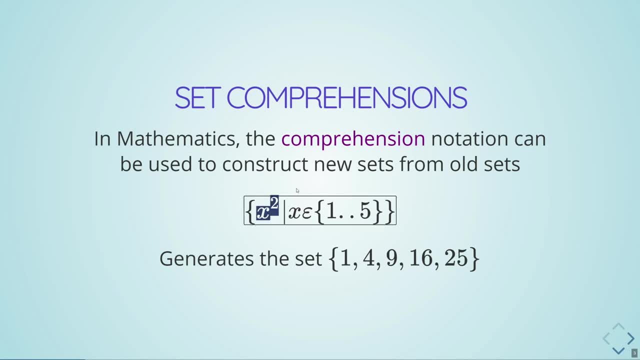 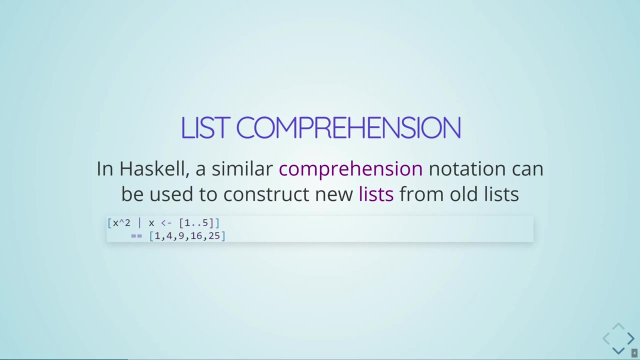 specify a new element, in this instance x squared. so this: we could use this set comprehension to generate the set 1, 4, 9, 16, 25. now, we shouldn't confuse lists as a data structure in Haskell to the abstract concept of sets in math. so let's go ahead and do that. so let's go ahead and do that. so let's go ahead, and. 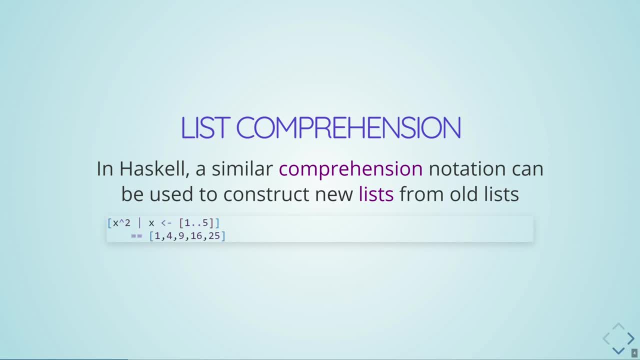 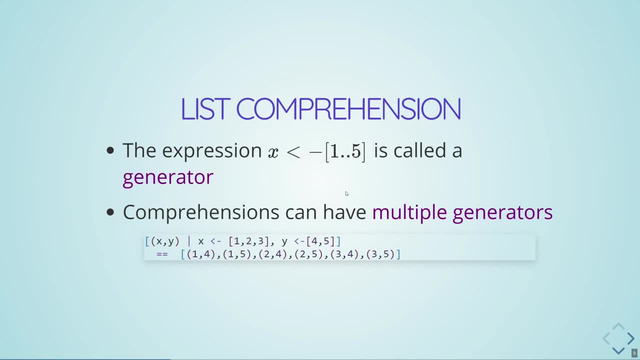 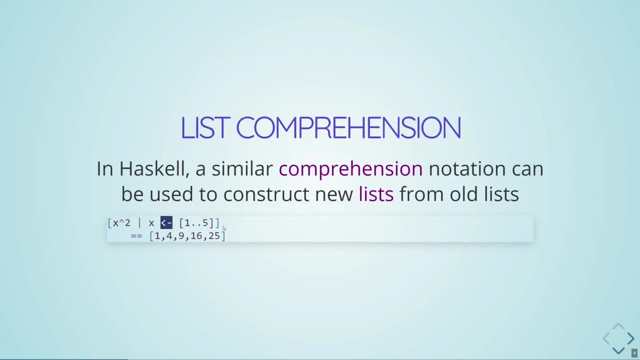 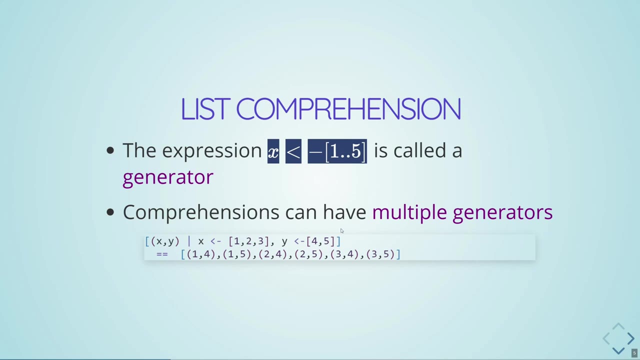 the x with an arrow part. okay is a bit different. so in mathematics we would say x is an element of the set. instead of doing element. we use this left arrow here and this part is called a generator. comprehensions can, interestingly enough, have multiple generators. so this comprehension has a generator for a variable x and a generator for a variable y. 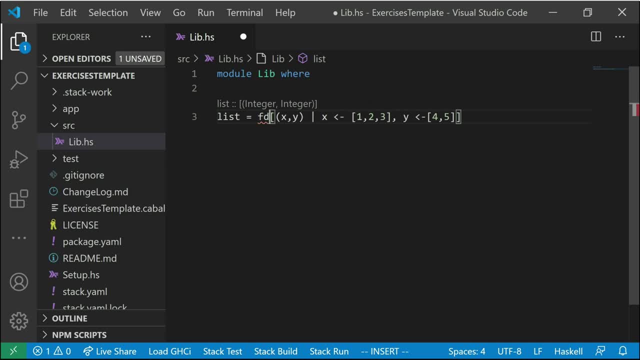 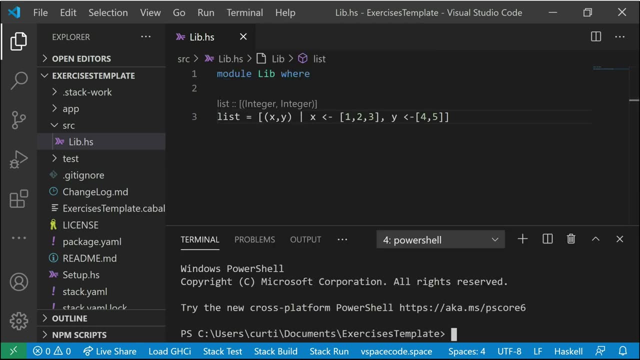 comprehension and ghci. so we'll assign the variable and load it into ghci. so make sure it's saved. open up a terminal and let's load this into ghci. hs, okay, and now let's run it list. so the resulting list: you'll notice that it iterates. it starts at x and iterates through y. 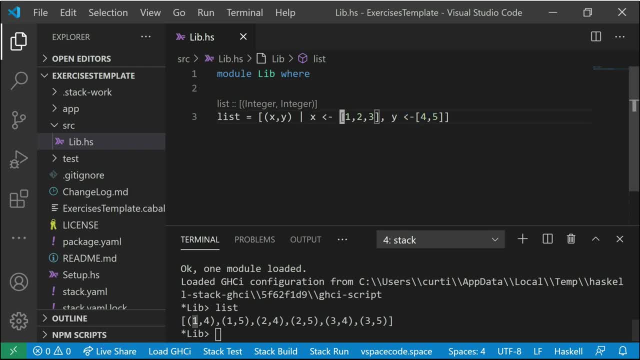 okay. so it's like: x is 1, so it starts at x, at 1, okay, and then the next element: it stays at 1, okay, and it's moving through y. and then when it gets through y, then it moves to the next element of x- 2, okay, 2, 4- and moves through like this. now let's say we um change these generators around. 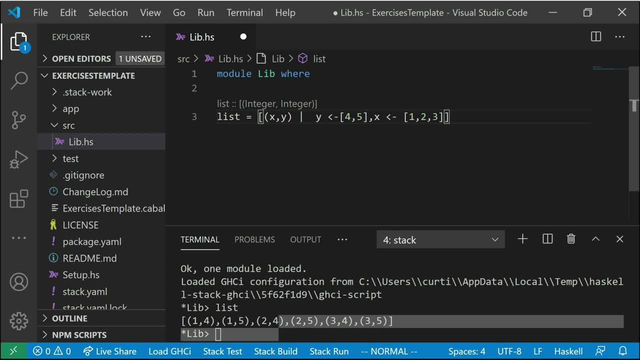 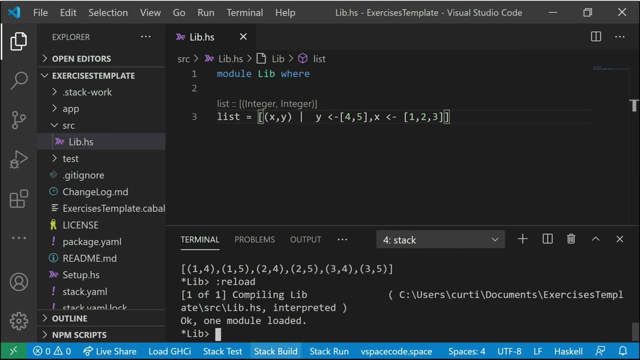 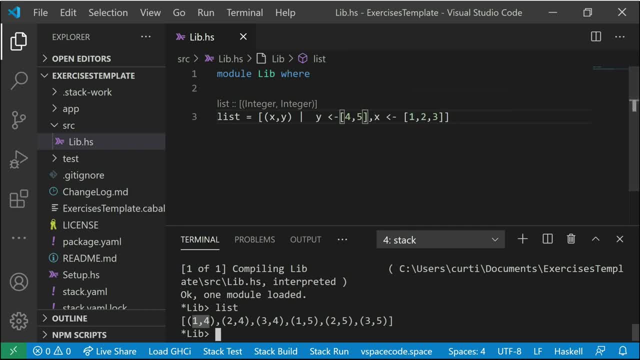 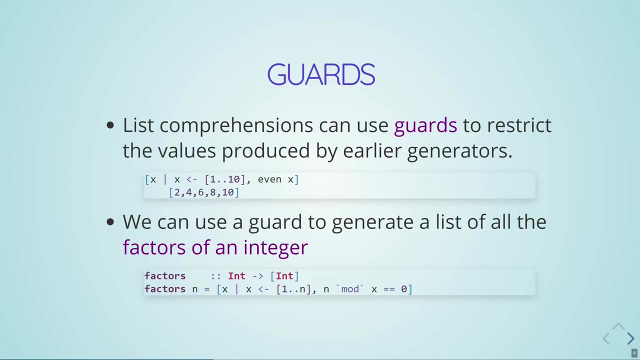 first. okay, so we're going to be. we're going to stick at four while we iterate through the x's. okay, so we start at four here, y stays at four, and then we iterate through all of the x's before we move to the next y at five. we can make our list comprehensions even more powerful by using something called guards. so basically, after writing our generator, 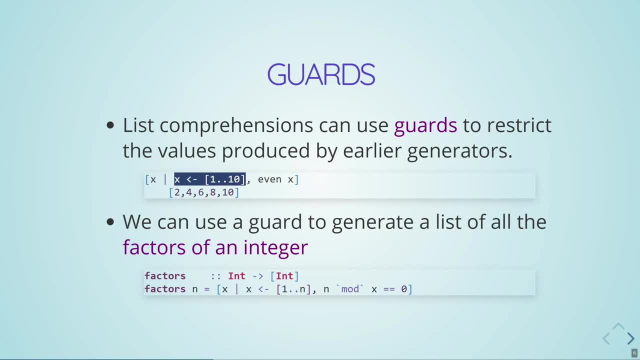 like inside this list comprehension here- where we have a generator that generates a variable x from 1 to 10, we put a comma and we could write any sort of Boolean expression that uses our newly created variable, And if the expression evaluates to true, then it will be included inside of the 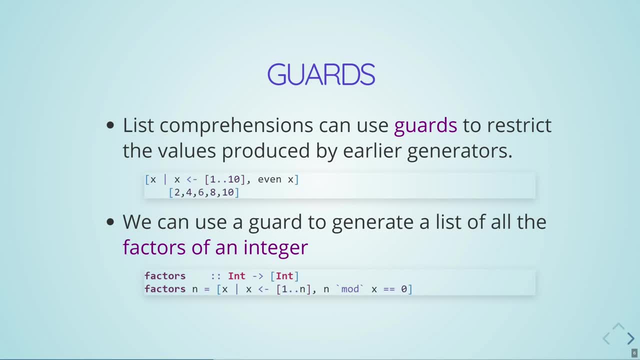 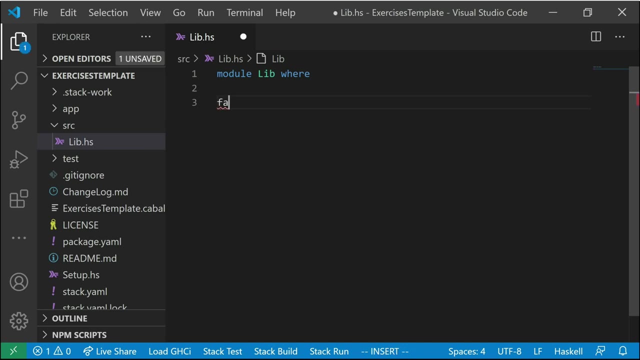 list. If it evaluates to false, it won't be included inside the list. So this way we could generate a list of even numbers by using the even function that only returns true when x is an even number. Another good example of this is if we wanted to find all the factors of a number n. 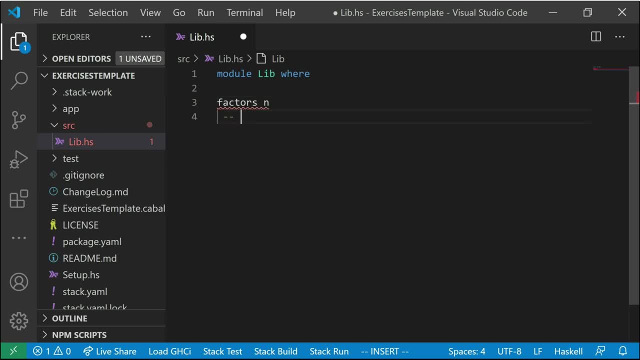 So the factors of a number- I'll put this in a comma here- let's say, the factors of the number six would be all of the numbers. okay, factors of six would be all of the factors of a number n, All of the numbers that divide six, and we probably want to exclude one. So one divides. 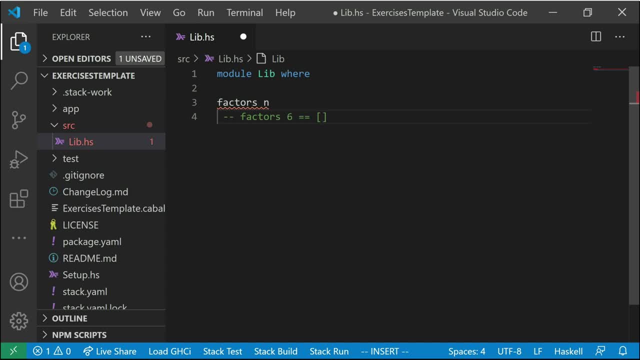 everything, So we can just exclude it. So two divides six, three divides six, four does not divide six, five does not divide six, six divides six. but we'll also exclude that, because every number is going to be divided by itself, And then, of course, nothing bigger than six is going to. 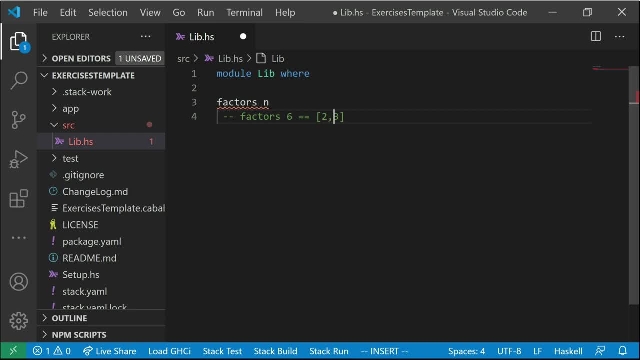 divide into six. So we're done. So the factors of six would be two and three. So what if we wanted to write a function that would generate this? so this is going to be a function. it's going to take an int and return a list event. 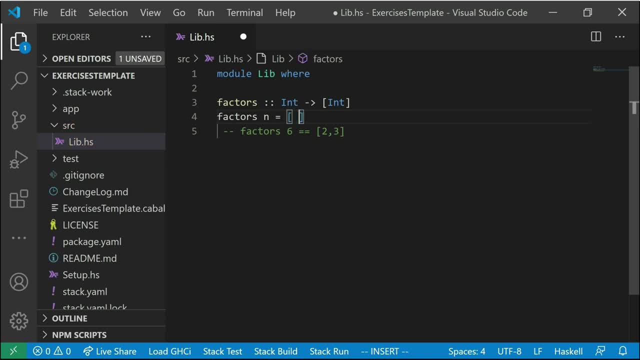 Okay, so how would we write this So well? we could do this with a list comprehension. So we'll generate x's and x will come from the list of. so we don't want to start at one, we'll start at two. 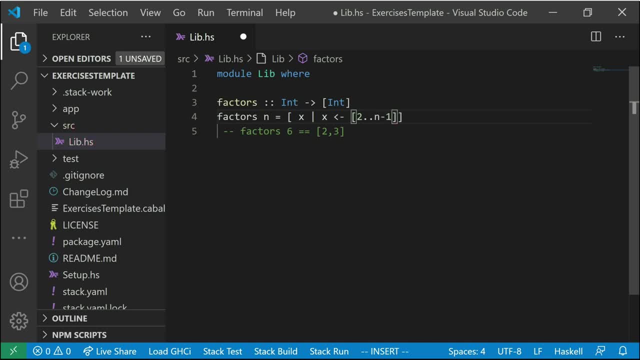 Two x or n minus one. Okay, so we want to. so these are all of the possible factors- will generate all of the possible factors of n. okay, so it'll be from two to n minus one And we'll say that n is. 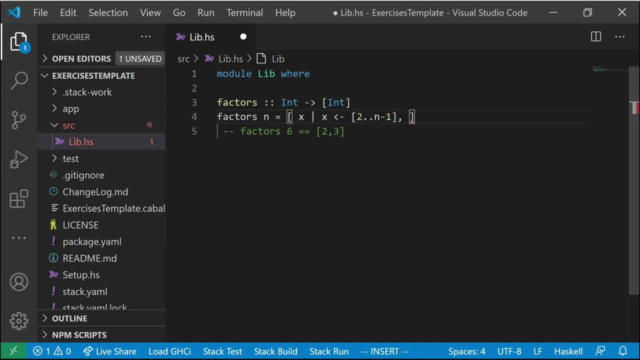 a factor, or x is a factor of n if n mod x equals 0.. So what is this mod thing? So let's load up GHCI and test it. So let's save it first and let's open up a new terminal. 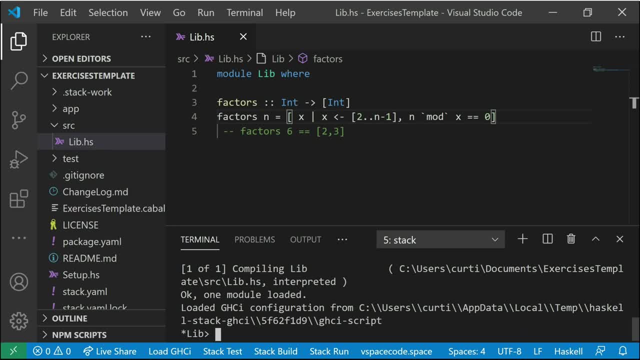 So I've shown you two types of division in Haskell already and I'll refresh your memory on them. So there's fractional division, So this is division with floating point numbers. So this is a division with decimal numbers. So that's just a simple backslash, the usual sort of division. 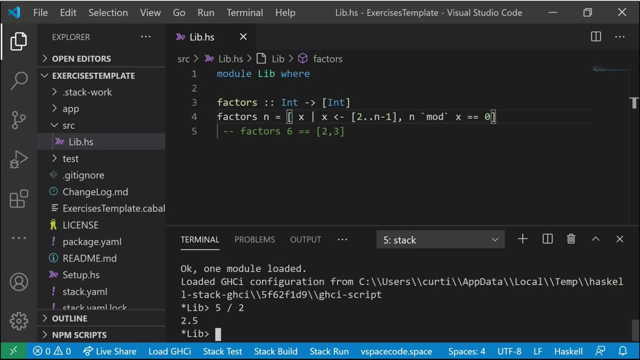 that you would probably figure you would enter into a computer. But then there's also integer division in Haskell, So this division will return the highest integer that gets returned. And now mod is a particularly useful operation. You see it sometimes in math, particularly in cryptography, but it's particularly useful in programming. 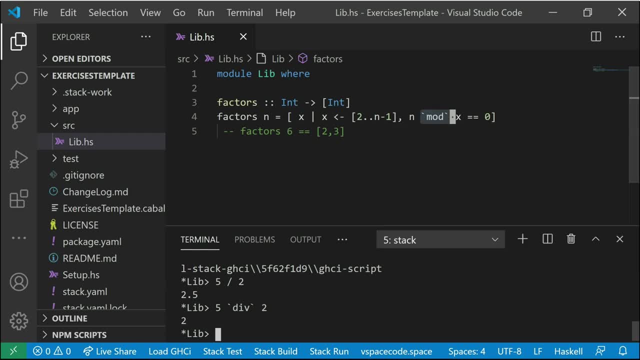 And it returns the remainder of an integer division. So you can actually put it over and it'll give you documentation of integer modulus. So this is actually the correct way you could formally define it. You see, underneath integer modulus satisfying that equation. So to give you an example, 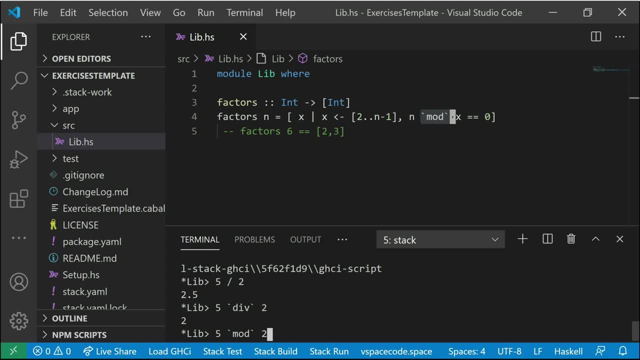 5 mod 2, what's this going to be? You guessed it: 1. Okay, because we try and divide 5 by 2 and it gets to 4. So it divides in twice. And then what's the remainder from there? 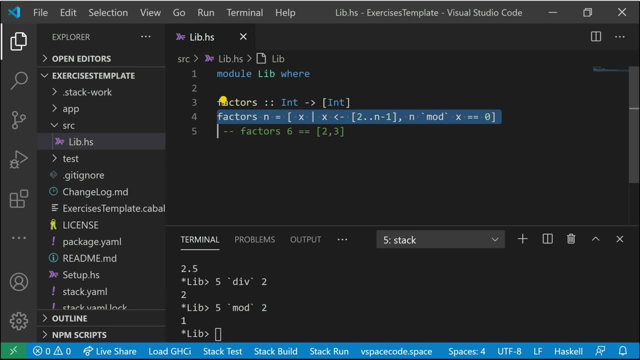 1. So our factors function. you could see something's going to be a factor of x. Okay, x is going to be a factor of n If x divides into it with no remainder. So I'm saying n mod x is going to equal 0.. 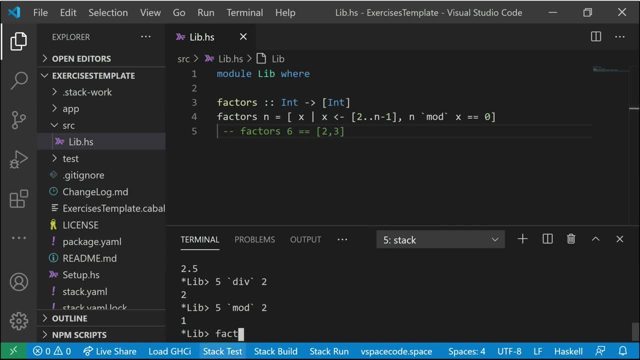 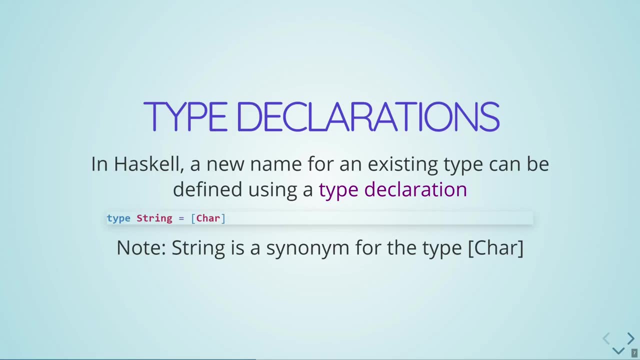 So let's double track that this works properly. Factors of 6. Yep 2 and 3. Now, without further ado, let's talk about how to create our own types. So the first way I'll explain about how to create your own type is with a type declaration. 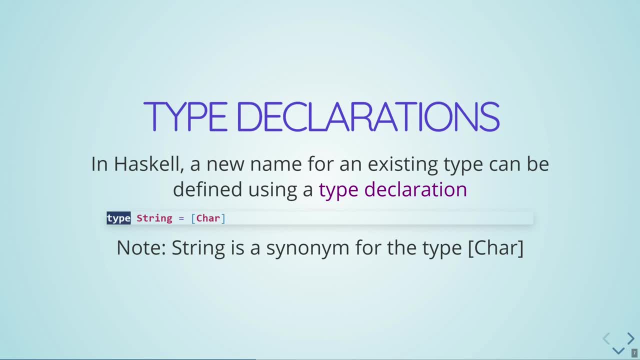 Okay, this is using the type keyword here, So I'll give you an example of a type that's actually already defined: the string type. So I've noted before that a string is actually just a list of characters and it has special syntax that allows you to use the double quotations. 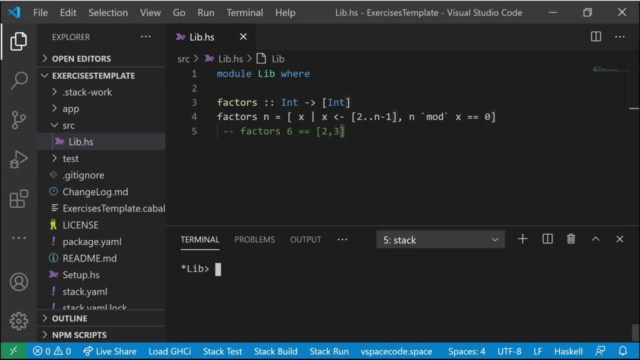 So if we go back to GHCI here, So a string just to illustrate this. let's say we have- So remember- characters. they need to be just a single character and they're put inside single quotes So we could have the list of single characters. let's say a, b here. 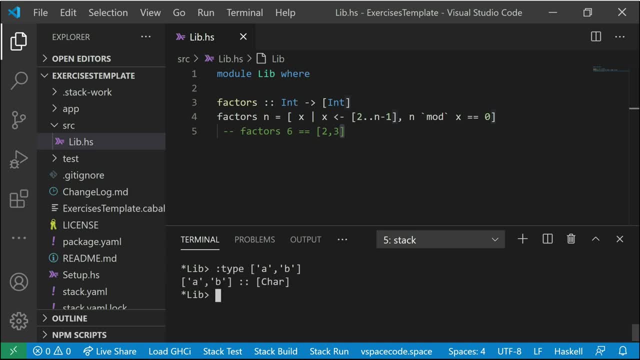 Okay, we could ask for its type. Okay, so this is a list of char, a list of characters, And you'll notice that this list of single characters can also be written using double quotations and just write the characters, as is Okay, so these are both the same thing. 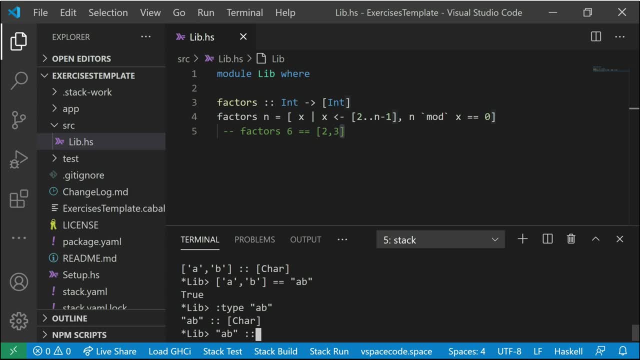 Okay, and just like I can specify that this is a list of char, there's a type definition in the prelude That was basically written like this: type string equals list of char. That allows us to use string in place of list of char. 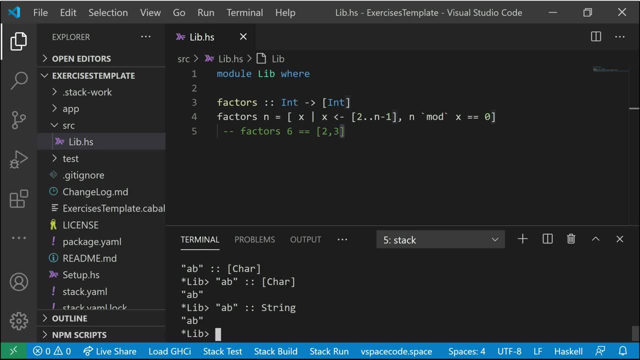 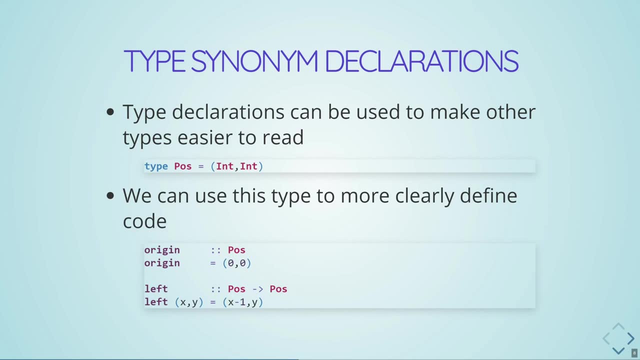 So another name for this is: we would call this a type alias or type synonym. So we should note: type declarations just give another name to something that already exists. So there really isn't any use in them except making your code more readable, your types more readable. 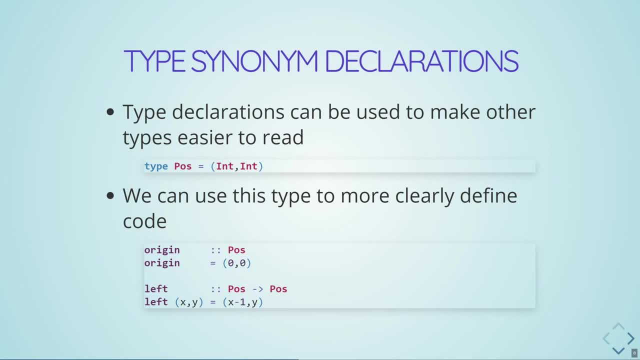 which is not something that should be underestimated. We do want our code to be very readable. This is a very desirable thing when programming. So a good example of this is: let's say we had a library that was plotting stuff onto a 2D screen. okay, 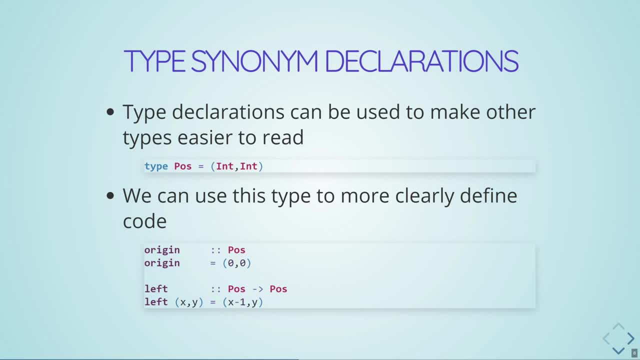 Like, let's say, maybe this is a library for doing 2D animation, So we would want this idea of a position on the screen. So what we can do is we could use a tuple in this example of 2-ents to specify the position on the screen. 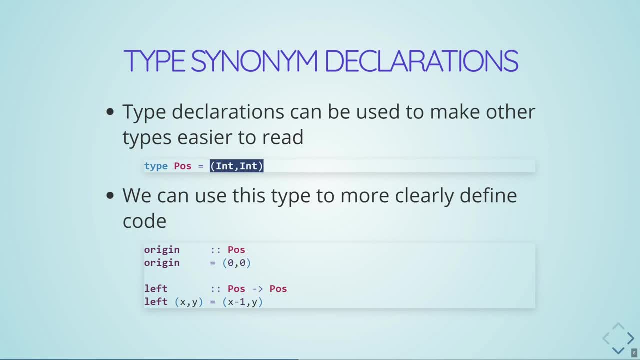 And just to make things more readable, to specify what this tuple of 2-ents is, we can make a type and give it the name pos for position okay. And then this way we could define different positions. We could say: oh, we have an origin, okay. 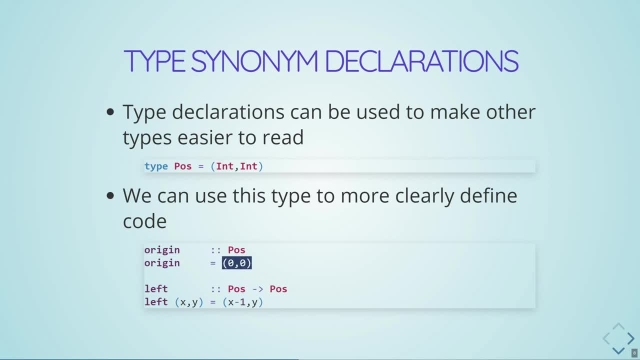 That would be the middle of the screen, which will be 0- 0, and then we could have a function left that takes a position and gives back another position. now, i mentioned this in the other tutorial. um, it's very, very nice to make it so that your functions, uh, are very. it's very easy to tell what they do just by looking at the name. 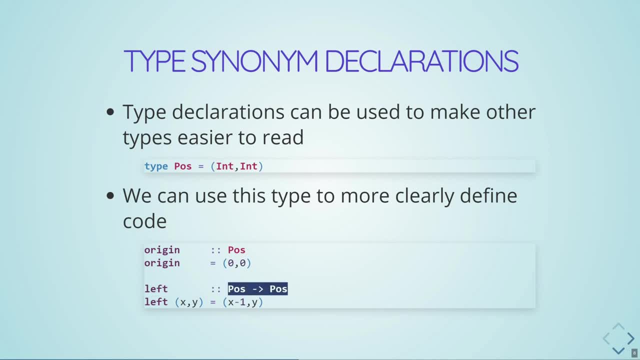 of the function and its type signature. this is why we put type signatures in our code. so this function- here left, it's called left- it takes a position and returns another position. what do you think it does? it moves a position to the left. okay, so, even though this is just for making things more, 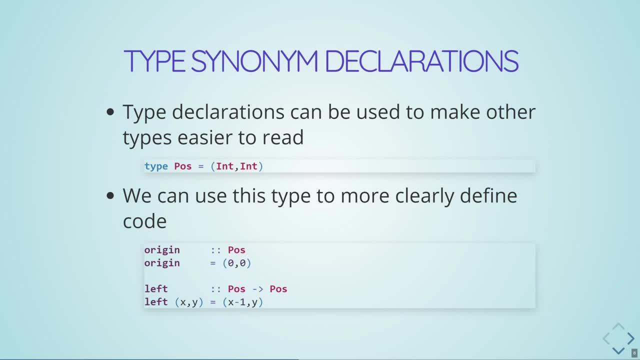 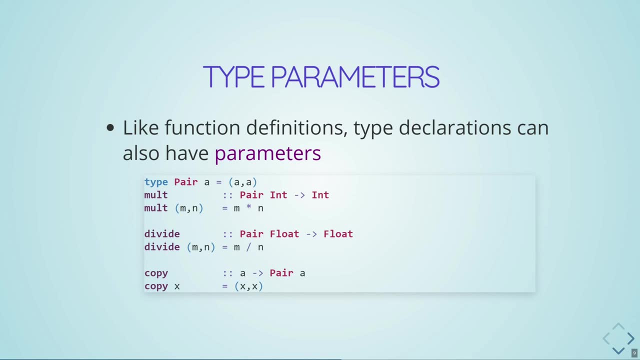 readable. you shouldn't underestimate it. it's actually a very useful thing in haskell now to make things a bit more interesting. type definitions can have parameters, just like functions do, so we could create a type pair that takes a type parameter, a. so note, just like with um, how i explained with. 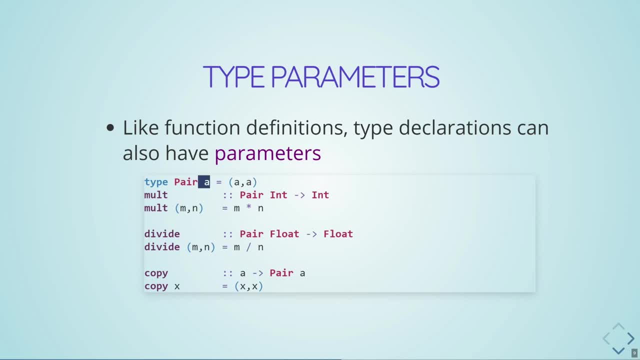 polymorphism. a is not a type itself, it begins. it's a lowercase letter, okay, and it doesn't have to be called a. i could have easily written the same thing with type pair. b equals the tuple of b, comma, b or type pair, you know anything, as long as there's a lowercase letter. 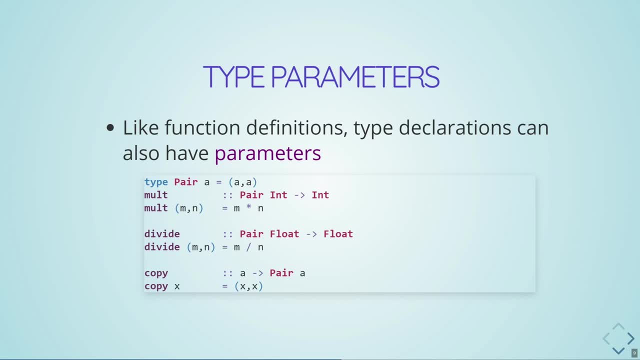 and in this way i can have a pair type that i then provide a specific type when writing a type signature when actually using it. so, um, this way my pair type. let's say i want to write a function that multiplies two integers together, given a pair of integers. okay, so this way i would specify: 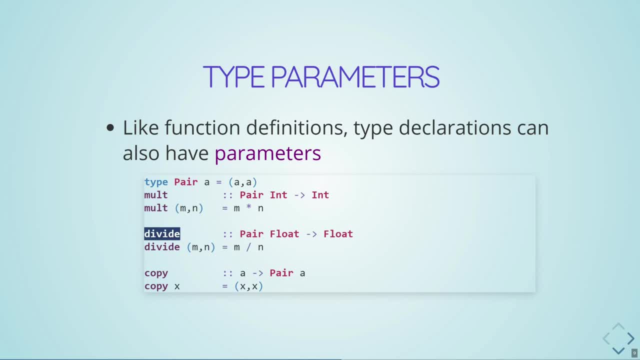 pair int. okay. or i could have a pair of integers and i could have a pair of integers and i could have a pair of integers and i could have a divide function that divides two floats together. or i can have a function that is polymorphic and doesn't specify the type. it takes any type, okay, a, and it creates a pair. it just 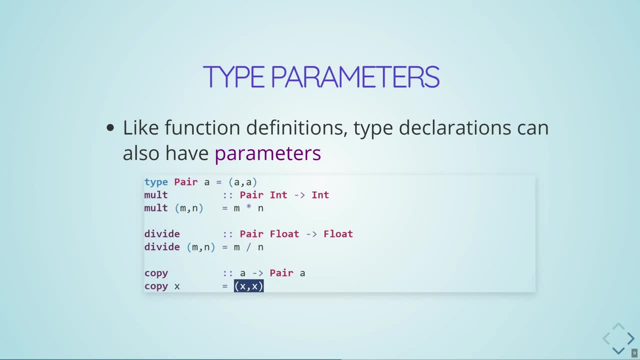 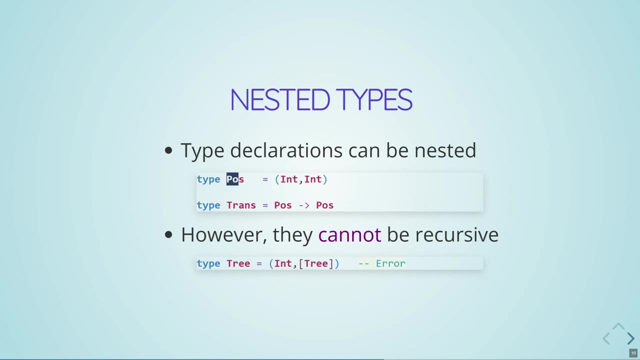 basically puts that type into a tuple. it takes its argument and puts the argument twice into into a tuple, so it creates another pair. a type declarations can be nested in that you can make a type declaration- let's say position- and then make another type declaration that uses that previous type declaration. okay, as soon, as soon as. 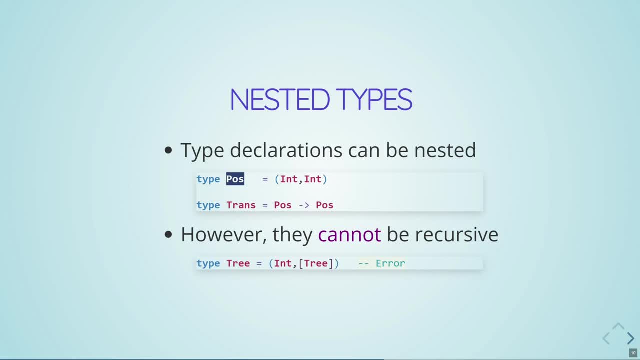 you make a type declaration. that's just a type like any other type in haskell. however, they cannot be recursive. so, um, we'll get into what i mean by this in the next tutorial coming up, coming right up. okay, but since i'm introducing types, uh type declarations to you now, i should 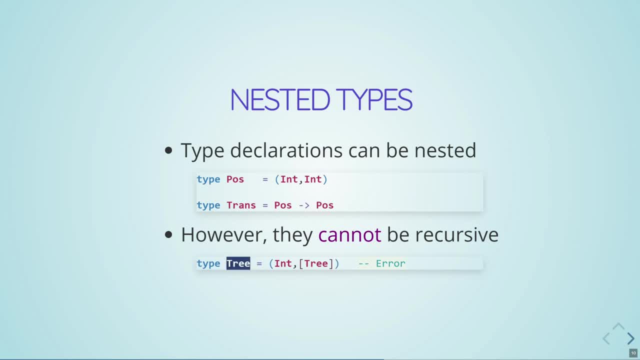 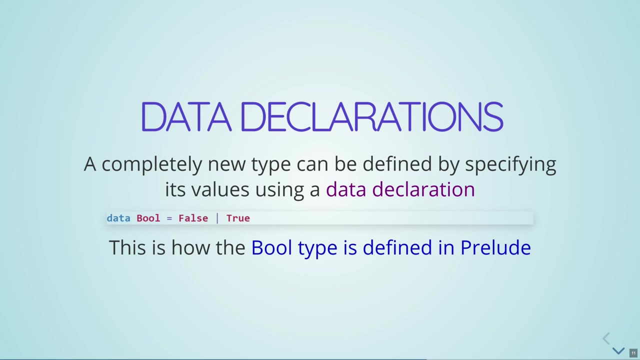 mention right now that you could not do something like this, where you declare a type tree and then in its own definition, you use that same type tree. data declarations are another way of defining your own types, but they're more powerful in that they actually let you create your own values. 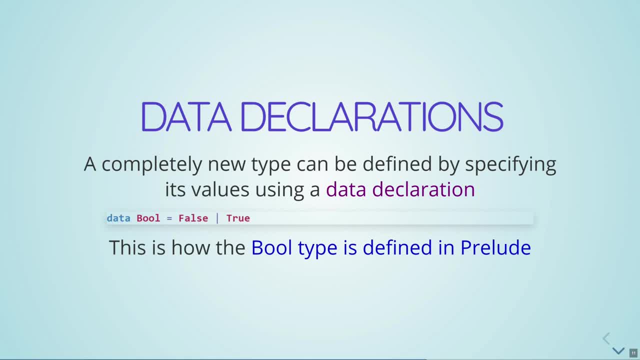 so type declarations: they don't create new values of any sort. they're just another name for a type and values that already exist, whereas data declarations they don't even. they don't just create a new type name, they create new values that are associated with that type. so, for instance, if we wanted to look at how bool is defined in the prelude, so the type. 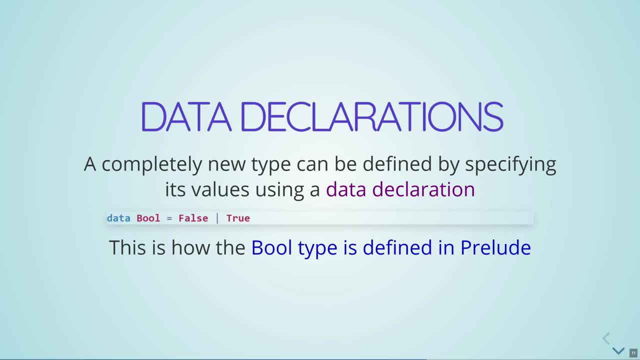 bool that we've been using all along. it's defined in the prelude and it's defined using the data declaration. data bool equals false and the way i like to read this is: or okay, you use this vertical bar, true. so basically, you specify all the values you want. 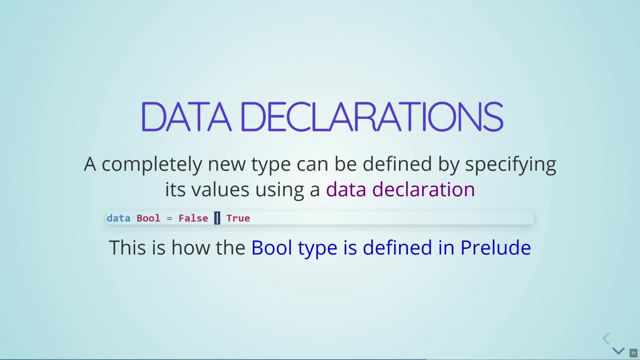 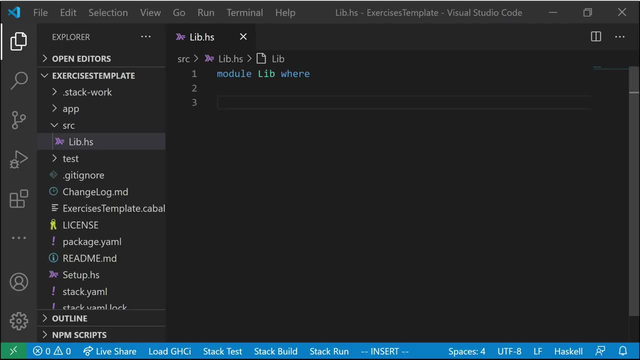 to be included inside of your data declaration, separated by a vertical bar. let's run through an example where we would want to create our own custom data type and not just use one that was already put into the prelude. so let's say we're um having a program that answers questions, okay, but the 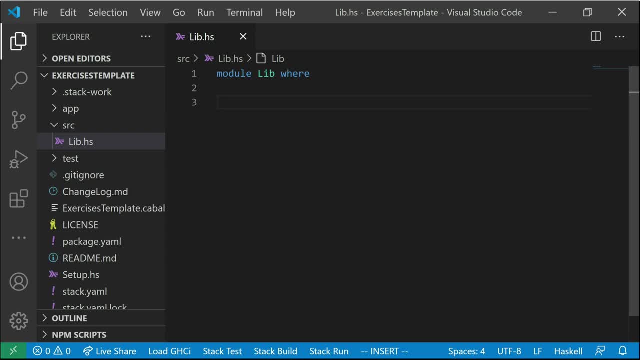 standard true or false answer to the questions aren't going to quite cut it. let's say we also want to have the option for a third answer of just i don't know. so we can create a data type. data answer equals yes or no or unknown, and make note here. okay, these are. 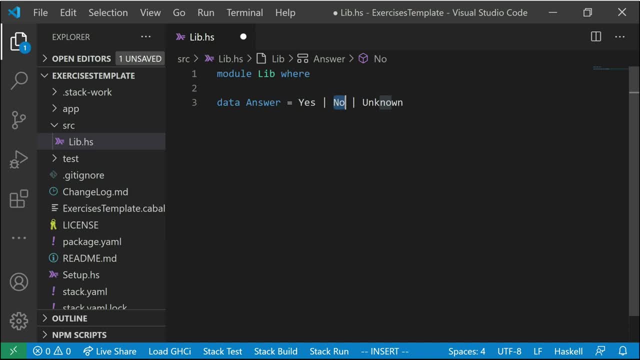 values that we're creating. okay, so they they need to begin with a capital letter, just like the name of the type answer needs to begin with a capital letter, and let's put this to you so we can create a function or let's just create a list. sorry answers. 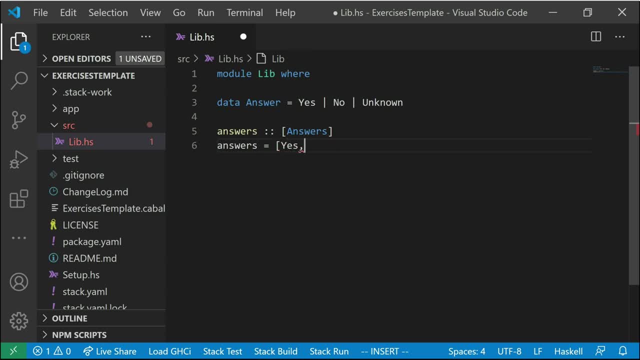 and answers are going to come out like this. so we're going to click on that and and i'm going to to consist of these three values: Yes, no or unknown. Okay, so we can go around and use these as values. Sorry, this is an answer. Use these as values, Just like we would use any other value. 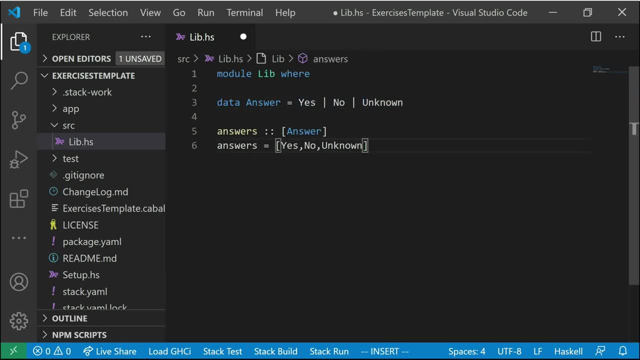 like true or false, or one, two, And we can create a function, flip, that takes an answer and returns another answer. Okay, And basically what this is going to do is flip will always just return the reverse of whatever answer you're giving. So if you give yes, it'll give back. no, If you give 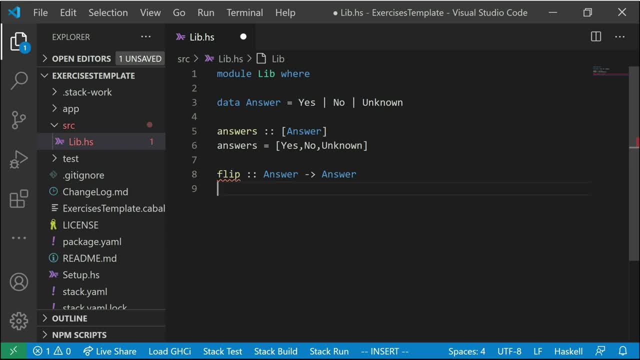 no, it'll give back yes, But if you give back unknown, it'll just stay at unknown. So the way we define this function is using pattern matching. So we'll, instead of writing like flip x equals something, instead of writing x there, we'll just put the value itself and define what the function. 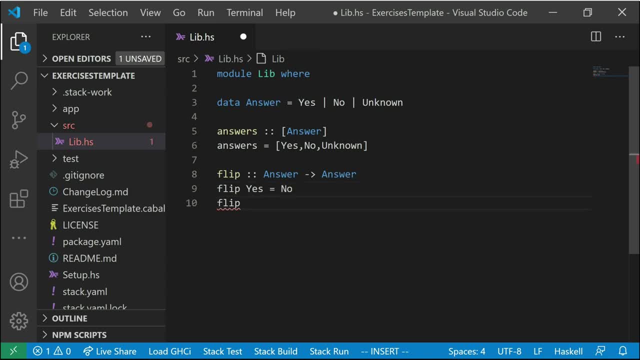 will equal at that value. So for yes it equals no, for no it equals yes, And for unknown it equals unknown. That's a little neat example. Let's try a another example. So we just let's say we're creating a library, that 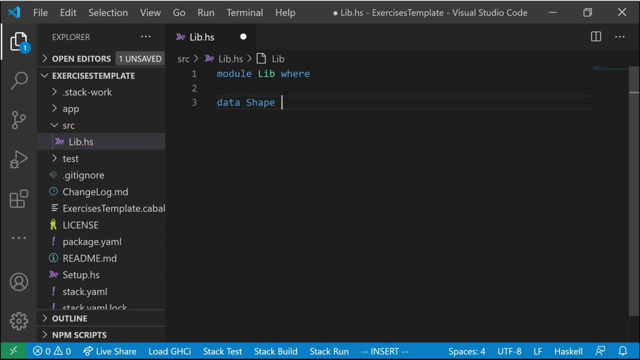 has to deal with different shapes. So if you create a data type for shapes and it could have values- circle or rectangle- But here's the thing, let's say we want to specify the size of the circles and the rectangles So we can give these values parameters. Okay, so for a circle we would want to. 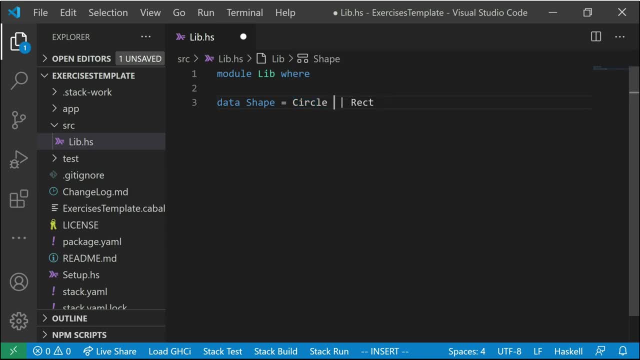 specify its radius So we can give it one parameter. So to do that, we'll put a parameter here And we're gonna have to have, we're gonna have to use another type for the parameter. So what would we want to represent? the radius, as we could do an int. but I think it makes more sense. 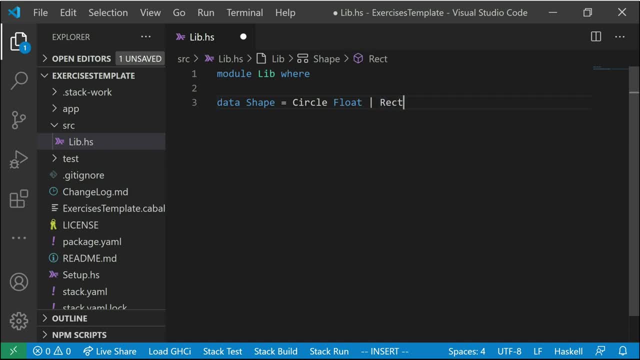 to do a float And then, similarly for the rect, we're going to want to specify the width and the height. So we'll give it two parameters to put space, float, float. Okay, so the way we would represent this now is we could have a square, so, like the units square would be equal to the rect of 1.0- 1.0.. So 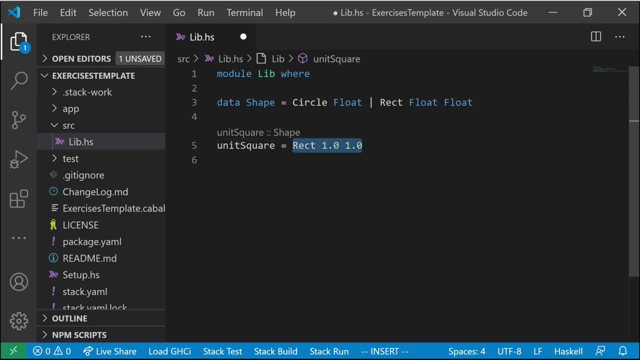 this is. this is how we were. we would have values of rep here, okay. so when we make the data type, we're saying, okay, this data type shape, so this is a thing of data of type shape. so this data type, it'll have name shape and its values will be circle with a floating. 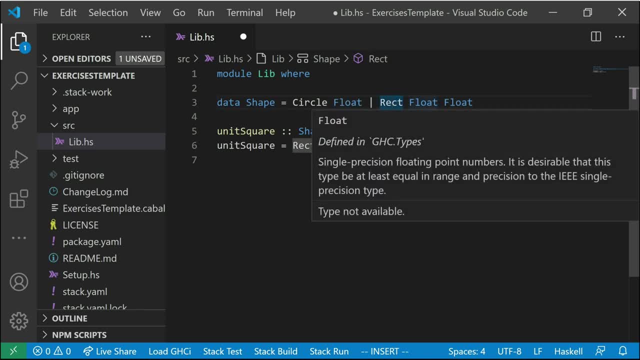 point value attached to it and or it'll be erect with two floating points attached to that. so, similarly, if we wanted to find the unit circle, that'd be circle 1.0. okay, and we could, we could define helper functions for this. say, we wanted to find, we wanted to define a function to construct a square. we. 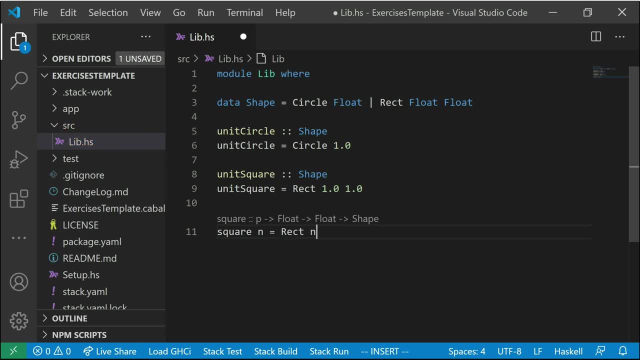 define a function: square n equals rect nn. so then, this way, instead of having to write rect 1- 1 here, we could just write square 1.0, and that'll construct a shape for us. we'd even define more interesting functions now, like, let's say, we want to define a 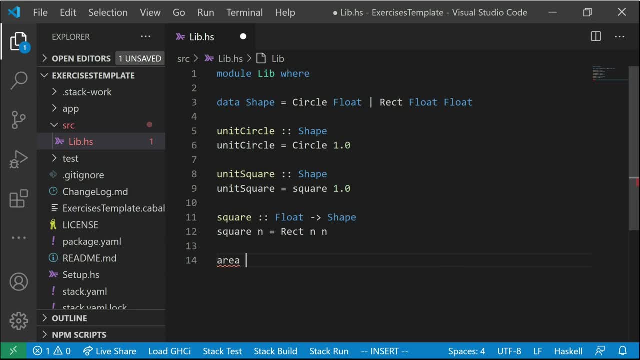 function that calculates the area of a shape. so this will take any shape, so that will include the circle or a rectangle and it will return a float for the area. so the way we define this, again we could use pattern matching. so there's two scenarios that we can match. 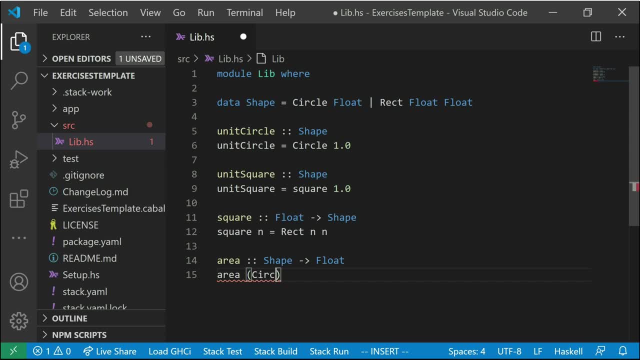 off of here. we could have a circle, okay, and that circle will have some float attached to it. so what we'll do is we'll leave a variable. we'll call it r for radius here. that will be the float that's attached to it and we'll say the. 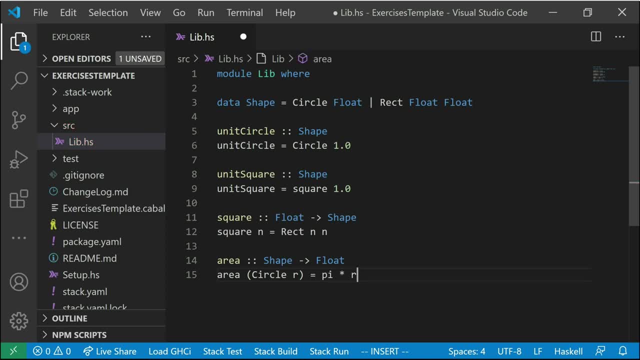 radius of a circle, if you guys didn't know, is pi times r squared, so that pi is a variable defined in the prelude. that's equal to an approximation of pi, so like 3.14, blah, blah, blah. there's no point memorizing beyond 1.4. and the other scenario is we have a rect, okay, and 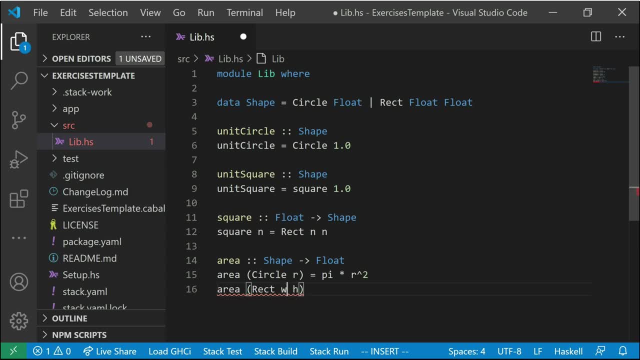 there'll be the width and the height of the rectangle, so we'll create two variables, w and h, that will represent these two floats here and the area of a rectangle is going to be 3.14, and the area of a rectangle is going to be: 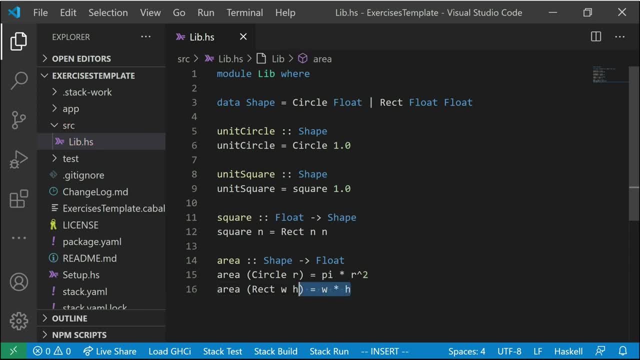 the width times the height. okay, so this way we can calculate the area of any circle or rectangle given to this function. a really interesting thing to note about the values circle and rect here, when they have a parameter attached to them, is that they're kind of functions on their own. so if we load up a terminal, 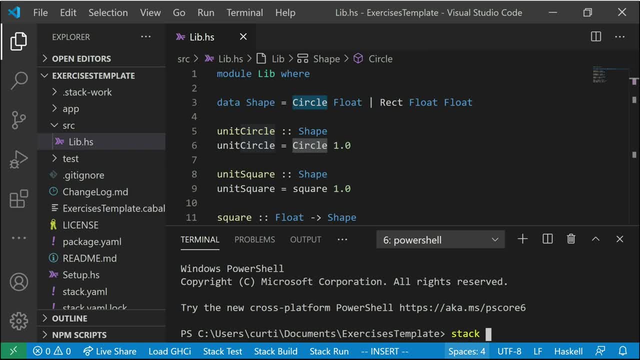 make sure this is saved and then we can see that we have a function that's called circle and rect and load this into GHCI. okay, and we ask it for the type of, say, a circle 1.0. this is a shape. okay, that makes sense. it's in the same. 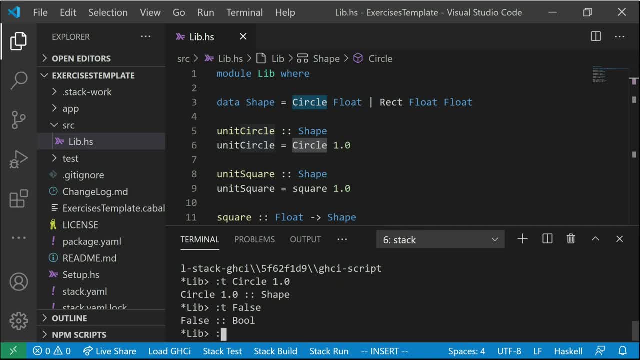 way that we asked it for the type of false. it's bool, right, but what if we asked it for the type of just circle on its own and we don't get the type of the circle on its own? and we don't get the type of the circle on its own and we don't. 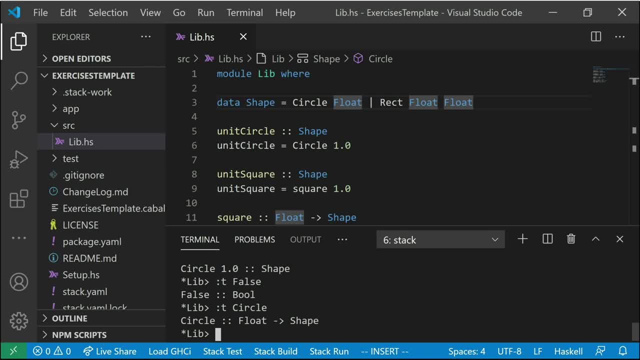 give it the float that's attached to it. well, circle is now. see, this is a function type signature, something that takes a float and then returns a shape. similarly, if we ask you for the type of rect, this is a function that takes two floats and returns a shape. interesting. 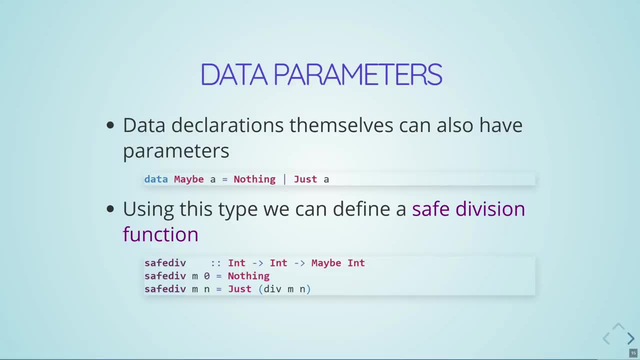 eh. one more thing I want to mention about data declarations before we finish off is that the function that takes a float and returns a shape is a function that takes a float and returns a shape is is Donald's React, but the function that takes a float and returns a shape二. I can add 쫍s to this and 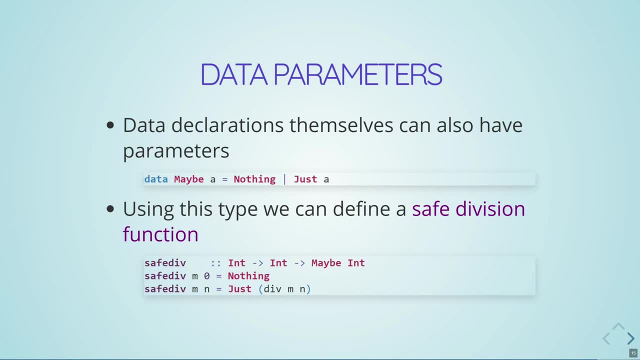 it's like another combination of Diego lunch update gave us a ducks so that we get a perfect form. just like type declarations, they can have parameters attached to them. so consider this type. maybe that get a perfect form, just like type declarations has a type parameter attached to it. so maybe it could either be nothing or 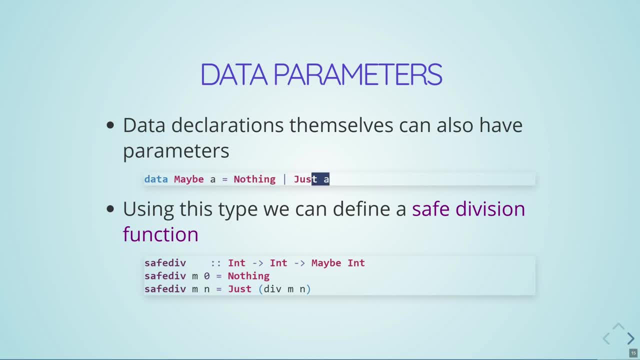 the answer to this one is the trap that I just made, so we need to take a but like type set up this again. just another: compression R is a text. if and 3D lại add Raw, please use red Seg Surfer to be host of this one. so 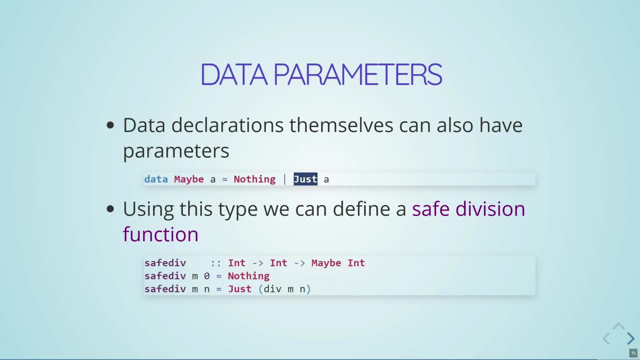 instead of being part of this next one, I can add barcode or something like this. but so Jest is a kind of function, just kind of like Valli ngec circle or functions that returns a value, of the type maybe, But unlike circle and rect that had a specific. 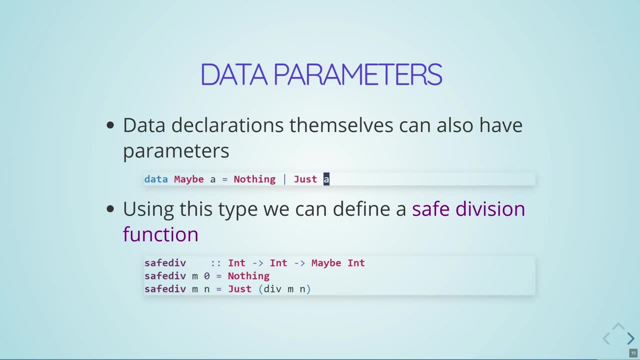 type attached to it. float just is going to have any sort of type attached to it, And whatever type it does have attached to it will reflect on what the maybe type itself is. So consider, for instance, if we wanted to define a function safe div, that instead of crashing when it tries to do division, 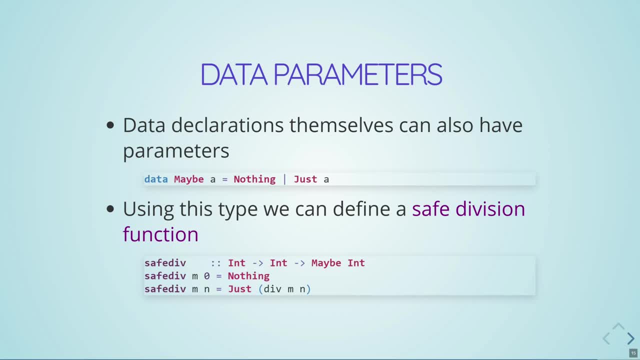 by zero, it returns nothing. So it takes two integers here, And if the divisor is zero, it just returns nothing. If it isn't zero, it's still. it can't just return the end in this case, because it needs to return the maybe type, right, So it returns just and then the end inside of just here. 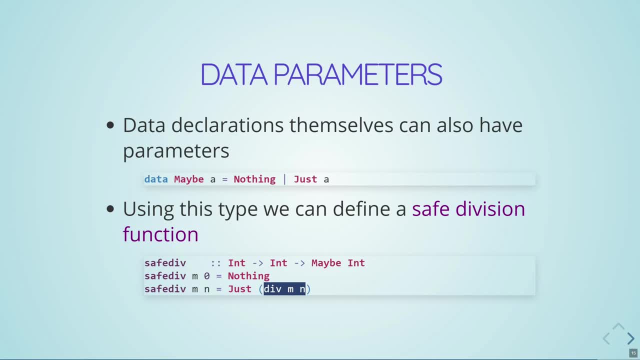 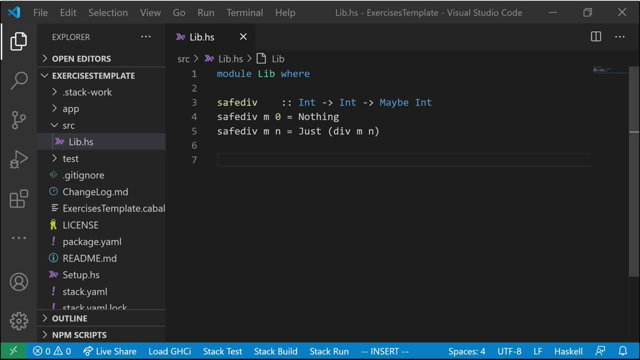 And then we get to find functions to pull that integer out if we wanted to, by pattern matching. So, for instance, let's say we have our function safe div, So we could first define a function to tell if we returned nothing, or just so we could say: is just, and if is just, is giving nothing returns. 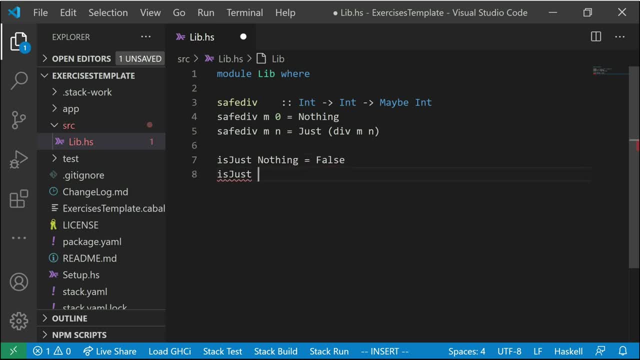 false And it is just is given just anything. So, remember, we can put this x or this underscore, for anything equals true, And then we can define, let's say, a list, comprehension div from 10.. Okay, it takes an n And what it does is: 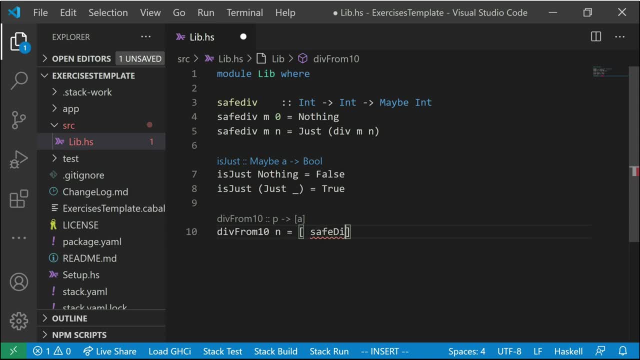 there'll be a list comprehension of safe div 10 x. okay, where x comes from. now let's see, I've got an x, a рез, half. Mommy dice l, unquote, z, function and dot dot. let's say: 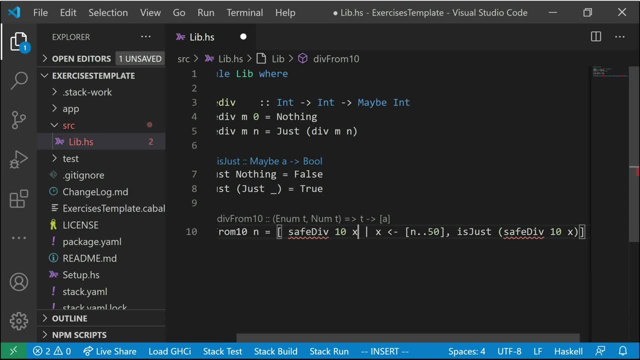 50. this is- this is a weird thing. so it's going to um use safe div here. oh, and i need to spell it correctly: actually save div. so it's going to use safe div here. i can put this on the line so you can see it. 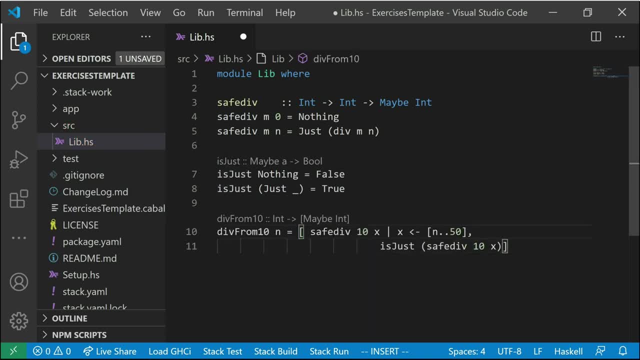 so it's going to create a list of maybe int- okay, but what it's going to do is it's actually has this guard here to be like. well, only include it if this result of safe div is a just right, and then what you could do is after you know, like you know, because you did this guard here. 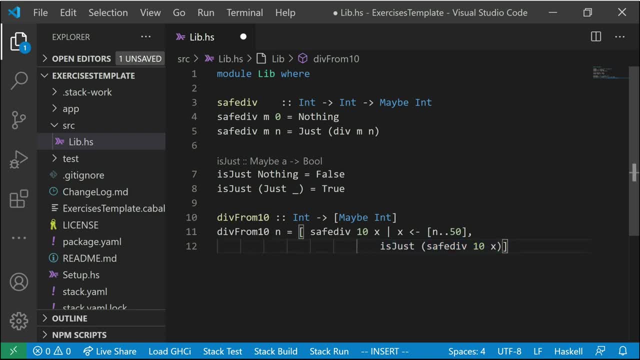 to tell that it's just after. you know this. you could define a function- we call this from just okay, where if it's nothing, then it throws an error, but then from just just x here, okay, it's going to return that x, okay, and then we could change this function. so right now, this will return a list of 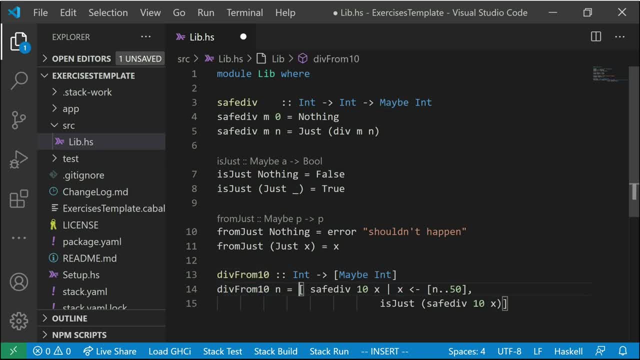 maybe int. so it's going to, it's going to basically return a list of just a bunch of like, just this, just that, and so on. so let's say we want it to actually just be ints, because now we know, because we're doing this guard, we know it's only going to return things that are just and never return. 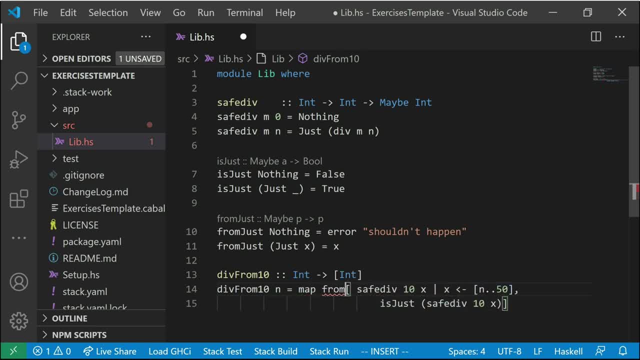 to nothing we can map from just over this list. so this is an instance where we've kind of um circumvented ever having to throw an error like this. okay, we're able to be like: well, we'll define the safe div that if division by zero happens, it returns nothing instead of actually 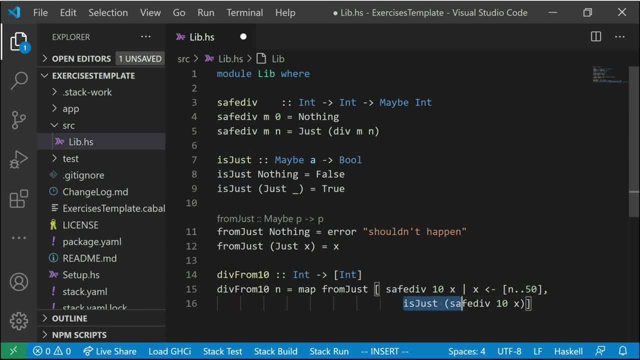 doing the division by zero, and then what we do is we filter out all of those instances. okay, because now we have this kind of wrapper around bad things that happen, and then we pull things out from that wrapper. okay, they, i'm calling it a wrapper, you could also. 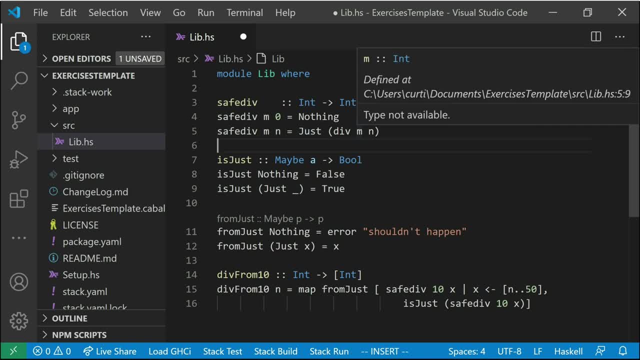 consider it the maybe type is kind of like a box, okay, where it's like it has a label on it of being nothing or just something, and you can put the actual values that you're concerned of inside of it. so this is a bit of a. this is a very interesting trick. i find that i think in haskell. 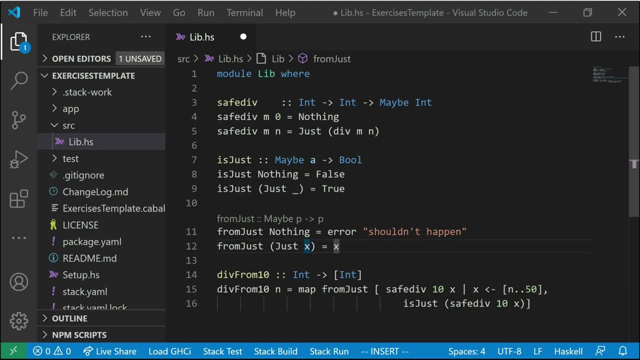 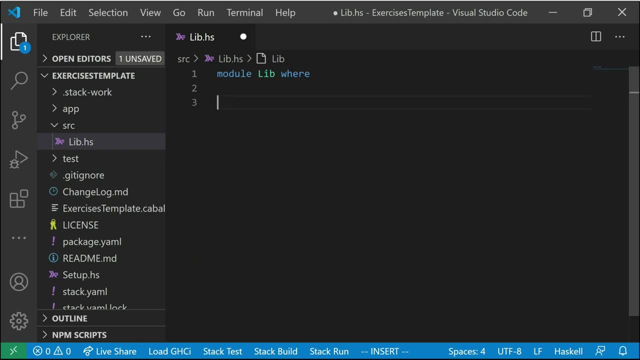 the other. um interesting example that we can do of this is, if you remember, at one point i mentioned how to find the function head takes x, x's or returns x, and i mentioned that the type of head: it takes a list of a and returns an a, as i was mentioning.